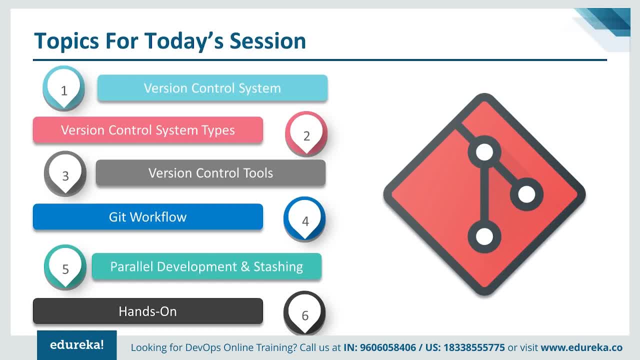 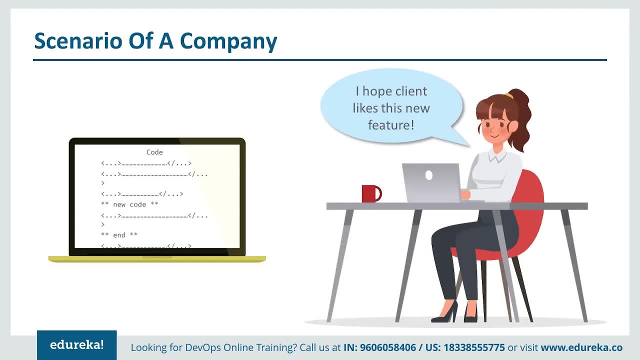 So is the agenda clear to everyone? Okay, So most of you have said yes, So now let's get started With the session. Let's consider a scenario of a company here. So Alice is a developer of a company and deals with deploying new features in the UIs created. 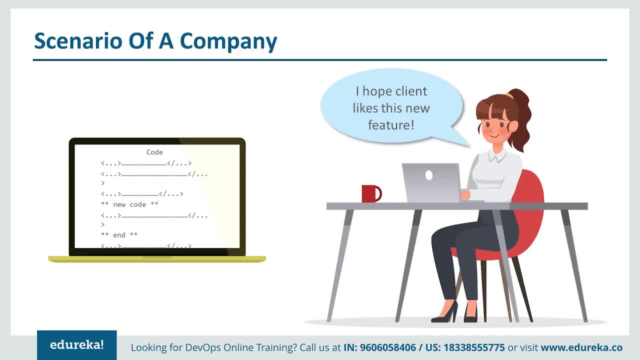 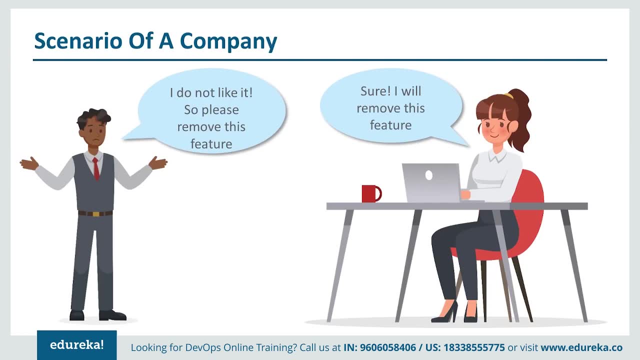 for the clients. So here she implements a new feature in the UI, hoping that her client would like it, But what happens is the client doesn't like the feature and asks her to remove the feature. So, as a result, she deletes the code. 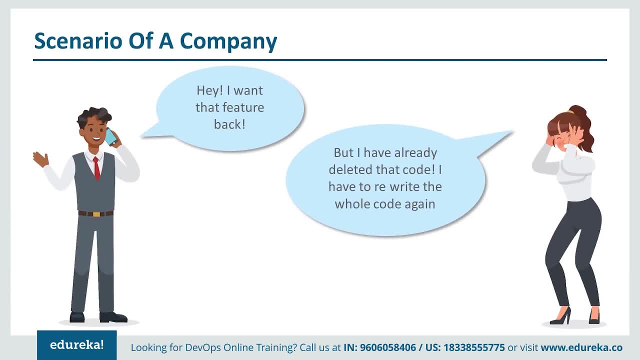 But after a few days the client calls her back and asks her to put the feature back. So now The company did not have the version control system. She has to do all the hard work again and then rebuild the code and then deploy it in. 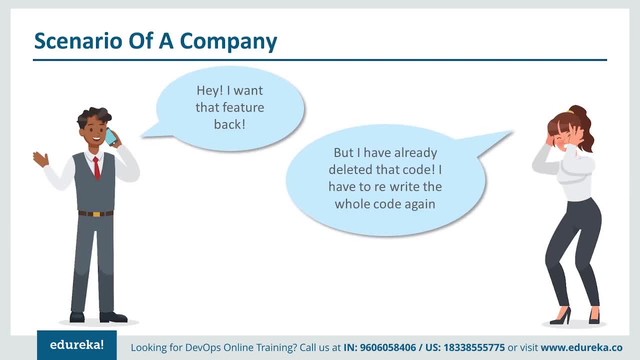 the UI design, but in such situations. So if the company had adopted the version control system, then Alice would not have to rebuild the code. instead, She would just pick up the code from the version control system and deploy it in the UI again, right? 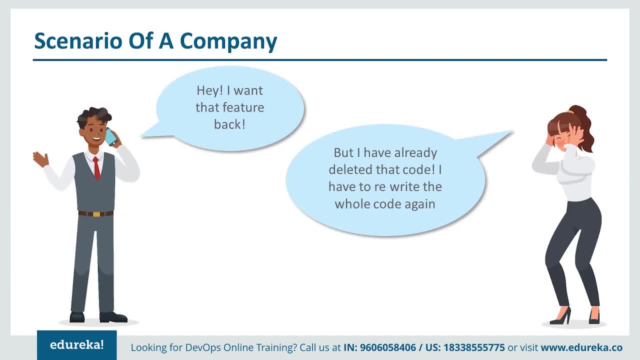 So wasn't it very simple with the version control system? It is right now. What exactly is this version control system? But before I tell you what exactly version control system is, Let me show you what was the chaos caused without the version control system. 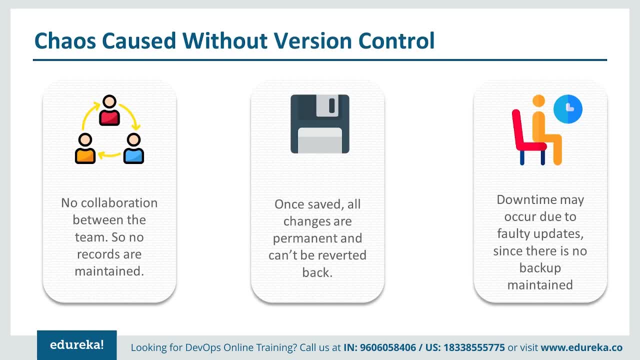 Well, without the version control system, There was no collaboration between the team. So basically there were no records maintained, Nobody knew who made the changes and where was the change made and when was the change made. so the team of developers working on a particular system made the changes by themselves. 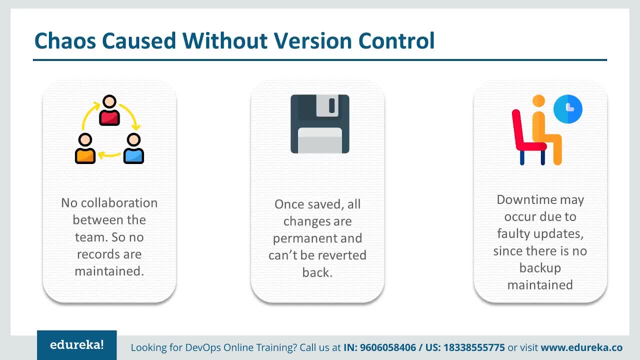 Now, secondly, once saved, all the changes are permanent And cannot be reverted back. So once the developer makes change in the code, then that change was permanent. Nobody could revert it back, even if it was wrong. So this was one of the main disadvantage of not having a version control system. 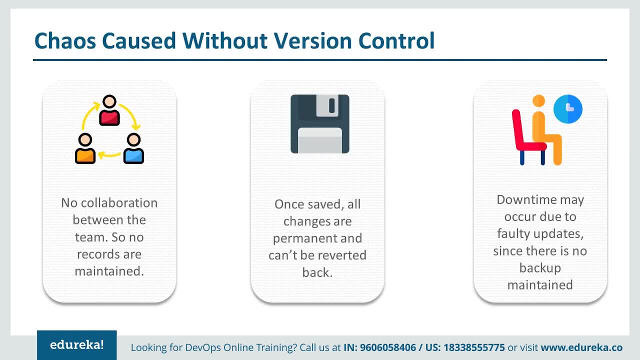 Not only this, but also downtime, also occurred due to faulty updates. that was because there was no backup maintained in any situation. if their code crashed in, the complete system would go down. So, looking at the above problems, Many organizations decided to come up with the version control system. 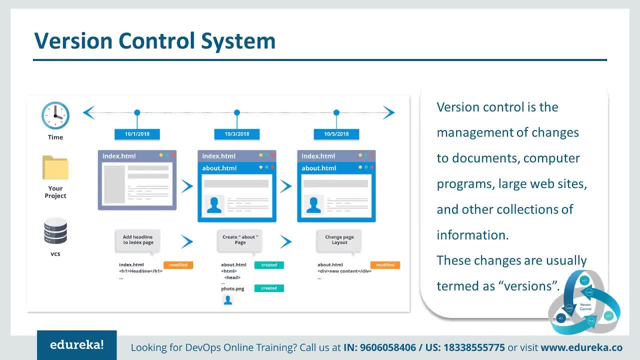 What exactly is version control system? Well, you can think of a version control system as the management system that manages the changes that you make in your project till end. So the changes that you make might be some kind of adding new files, or you're modifying. 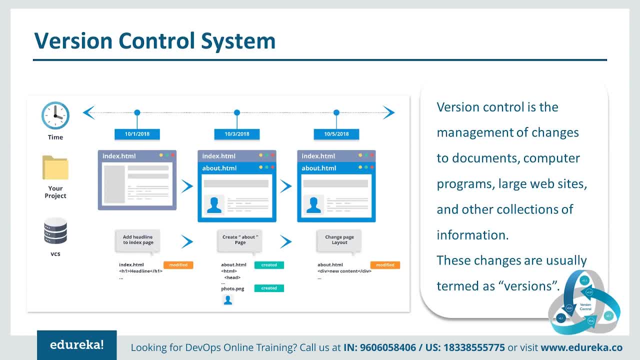 your folder or it could be any kind of changes, right? So what the version control system does is that every time you make a change in your project, it creates the snapshot of your entire project and saves it, and then these changes- snapshots are known as versions. 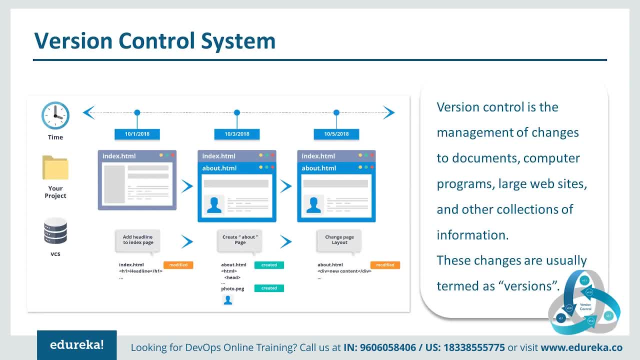 Now, if you have a problem with the word snapshot, just consider that snapshot is actually the entire state of your project at a particular time. That means it will contain what kind of files your project is storing at the time and what kind of changes you have made. 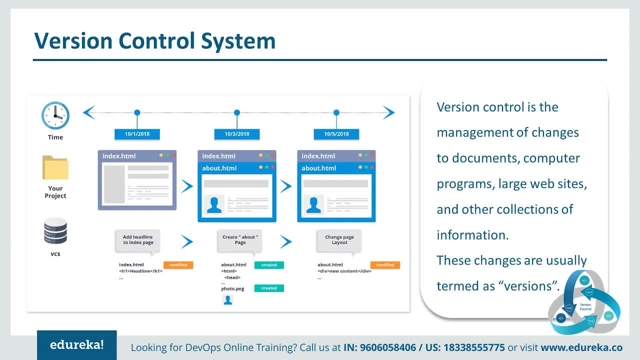 So this is what a particular version contains right now. if you see an example here, let's say that I've been developing my own website. So let's say in the beginning I have a web page as indexhtml. after some time I add: 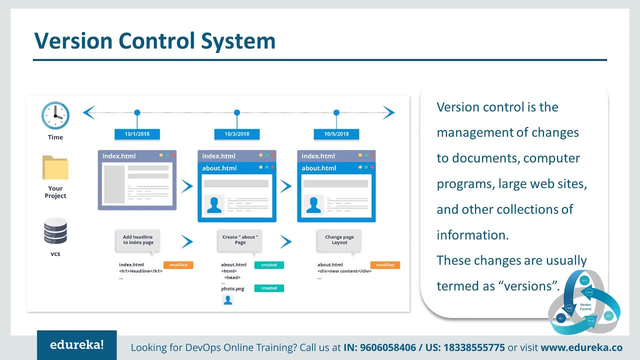 Another web page of about dot HTML. So in this about dot HTML, let's say I've added some kind of pictures and some kind of text, right? So what exactly the version control system stores is that it detects that something has been changed, right? 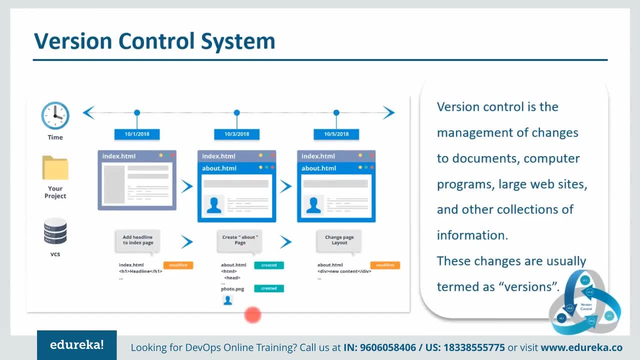 Something has been modified. For example, if you see here in the about dot HTML, it is showing that a photo has been added. So let's say that after a few days I've changed the entire page layout of about that HTML. So again with the version control system. 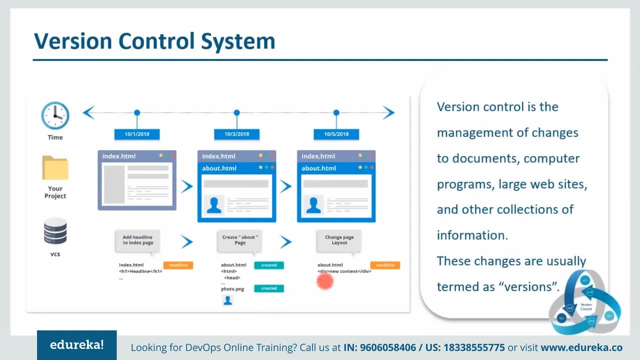 We will detect that some kind of change has happened and that will say that about dot, HTML has been modified and you can consider all these three snapshots as different versions. So when I only have my indexhtml and I do not have any other web page, 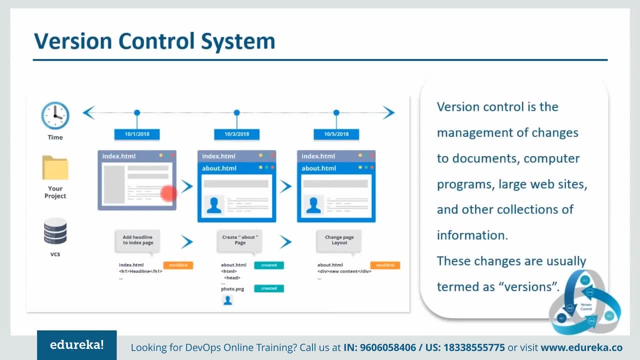 This can be considered as my first snapshot and then, when my about dot HTML has been created and some photos have been added, This can be considered as my second snapshot. in the similar way, Once the abouthtml HTML has been modified- that, that is, the complete layout, has been modified- that can be considered. 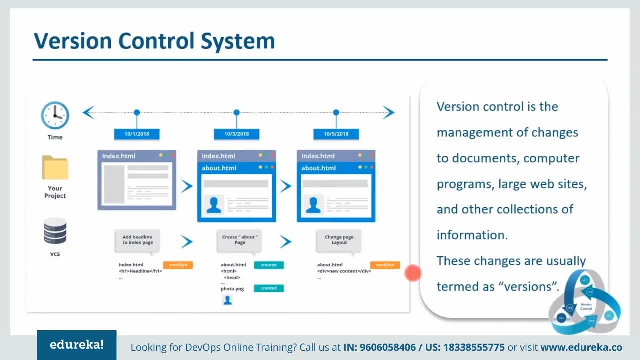 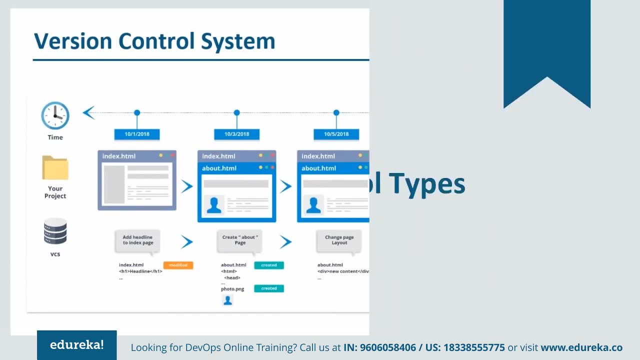 as my third snapshot. So the three snapshots could be identified as version 1, version 2 and version 3.. So, guys, this was basically how a version control system stores different versions, So I hope that you've understood what our versions and what is version control system. 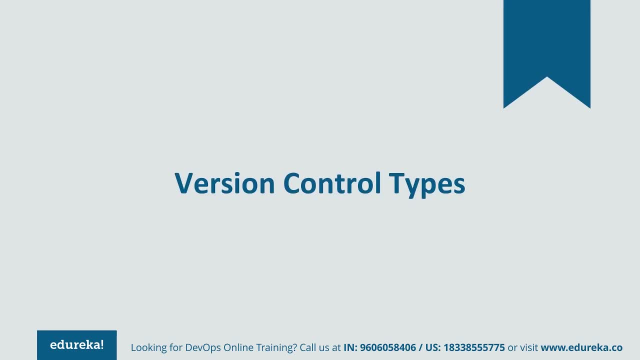 Let's get into the different types of version control system. Well, to say that there are three types of version control systems: The local version control system, the centralized version control system and the distributed version control system. So when you talk about local version control system, the local version control system is: 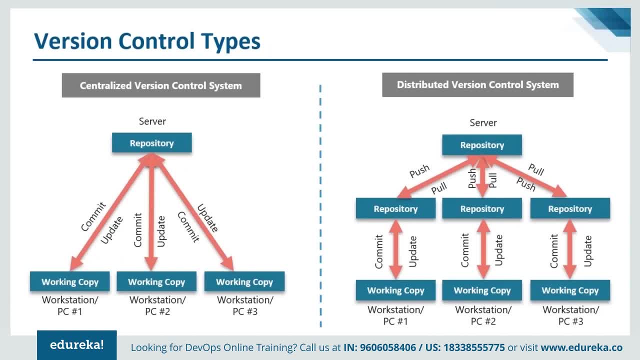 where many developers are working on the same version. now coming to the centralized version control system. centralized version control system consists of a central server, So it basically Stores all the files and enables team collaboration. It uses a central repository which stores all the files in that repository. 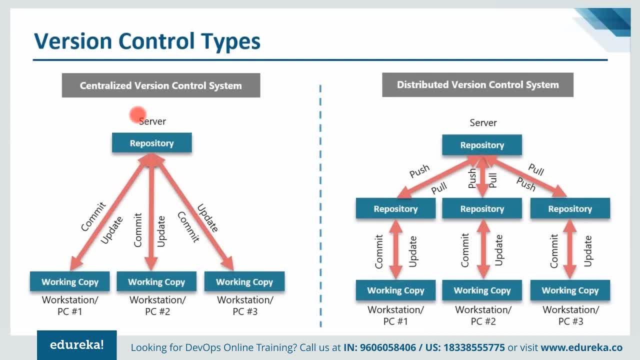 So that users can and accesses. So this is what happens here, guys: Every developer has a working copy. If there are n number of developers working on a single repository, then there are n working copies. the moment they want to make a change in the source code. 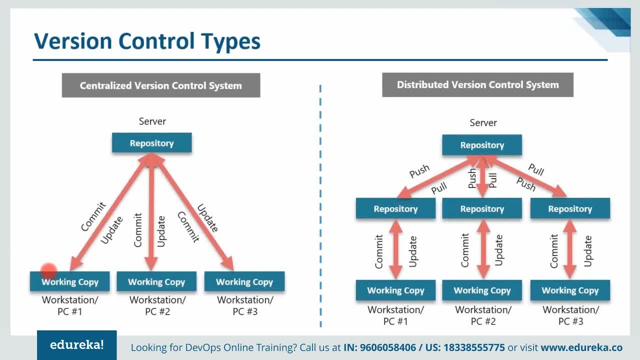 They can make change in the shared repository and then they can also update their working copy by pulling their code from the shared repository to their working copy. So the repository that you see on the screen indicates a central server that could be local or remote, and is directly connected to each. 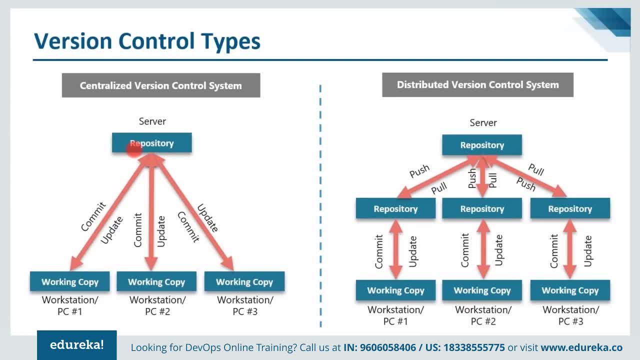 of the programmers workstation. So the central repository is connected to each and every working copy. now every programmer can extract or update the workstation from the code present in the repository, or can even make changes to the data or code present in the repository. So every operation is directly performed. 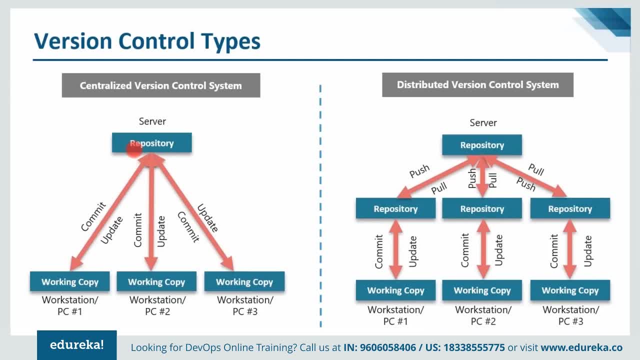 on the central server. Now, this may seem very convenient to maintain a single repository, but it has many drawbacks. before I tell you what are the drawbacks, Let me tell you what advantages it provides. So every time you come it, there will be a commit ID associated. 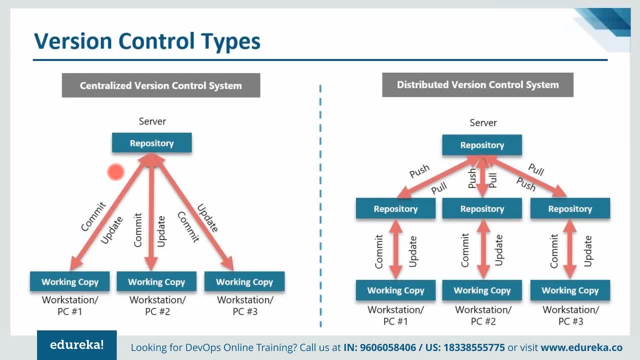 to it and also there will be a commit message associated to it. So basically you know who is making the commit at what time and what has been changed in the code, So you can always revert back to that particular commit and then make the changes again. 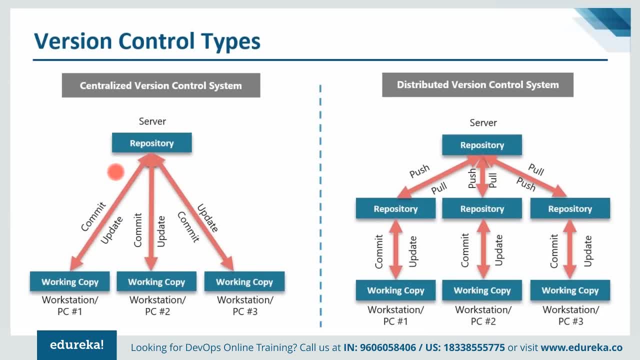 Now let me tell you some disadvantages about centralized version control system. First of all, it is not locally available. That means you always need to be connected to a network to perform any action, since everything is centralized. So just in case, because of any calamity, the central server goes. 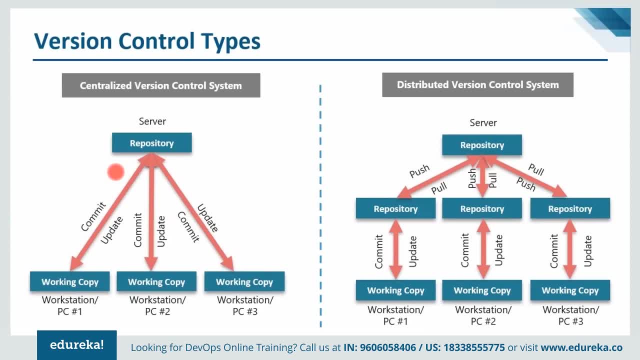 down, then it results in the loss of data for the complete system. This was one of the main reasons why centralized system is not used in many Industries. Now let's talk about distributed version control system. Now, these systems do not necessarily rely on central server. 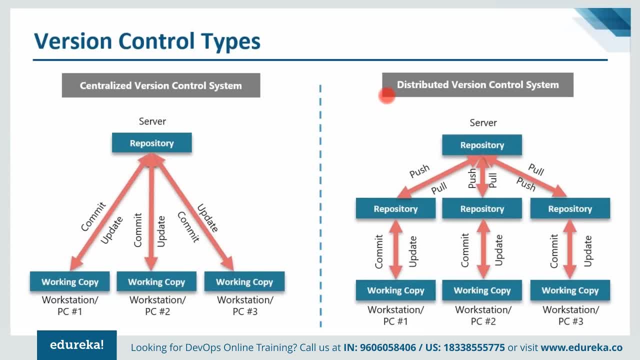 to store all the versions of the project file. So in distributed version control systems every contributor has a local copy, or the clone, of the main repository. that is, everyone maintains the local repository of their own and then contains the files and the metadata present in the main repository. 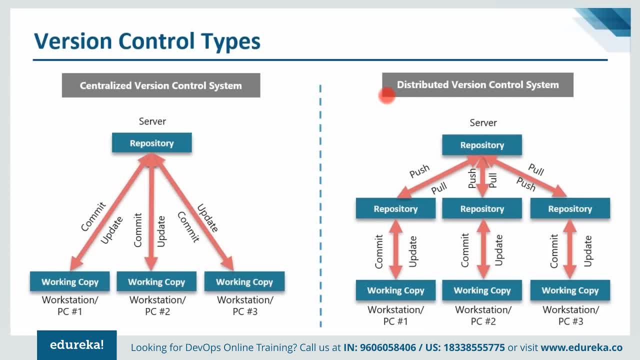 So, in simple terms, everybody has a copy of the remote repository. as you can see in the diagram, Everybody maintains a local repository on their own and they can come it and update their file without any interference, right? So they can update the local repositories. 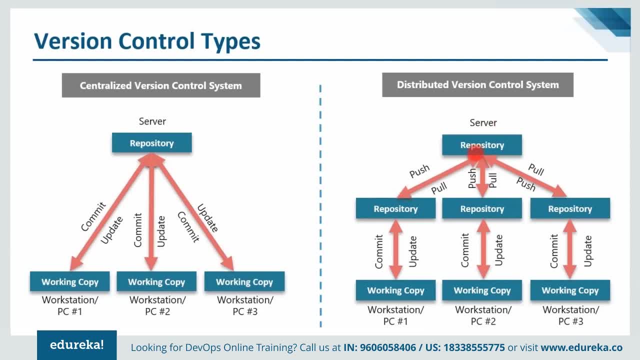 with new data coming in from the central server by an operation called pull and then affect the changes to the main repository by an operation called push right. So if you want to pull the data from the remote repository to your local repository, then you use the pull operation. 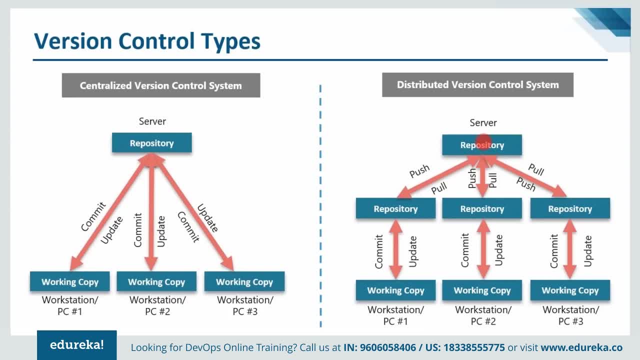 And then if you want to make the changes from the local repository to the remote repository, then you use the push operation right. So now that I've told you what centralized and distributed version is, all of you might be thinking on the advantages of distributed version control. 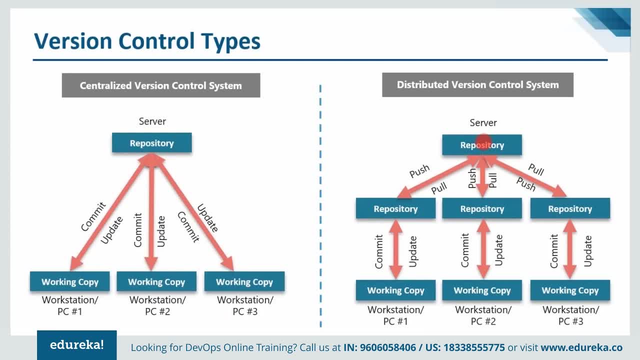 over the centralized version control system. So basically, act of cloning gives you the main advantage. So now let me tell you how all operations, apart from push and pull, are very fast because the tool only needs to access the hard drive and not the remote server. 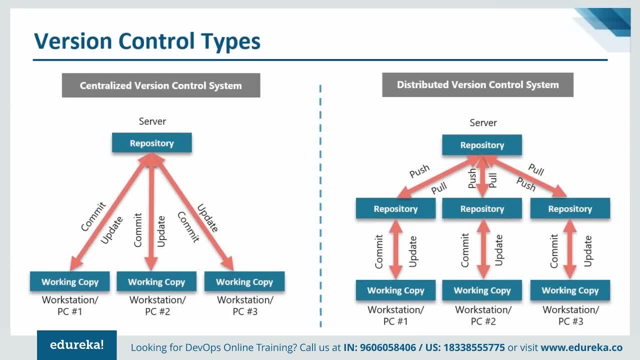 So with this functionality, you do not need the internet connection always. now committing new changes can also be done locally, without manipulating the data on the remote repository. So just in case, if you want to make any changes, you can take feedback from the other developers. 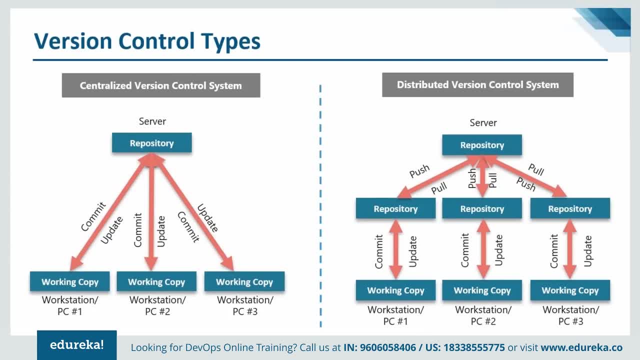 and then, once you make the changes, you can review them once and then push those changes to the remote repository. Now, if the central server gets crashed at any point of the time, then the lost data can be recovered from any of the local repositories. So this was not the case in the centralized version. 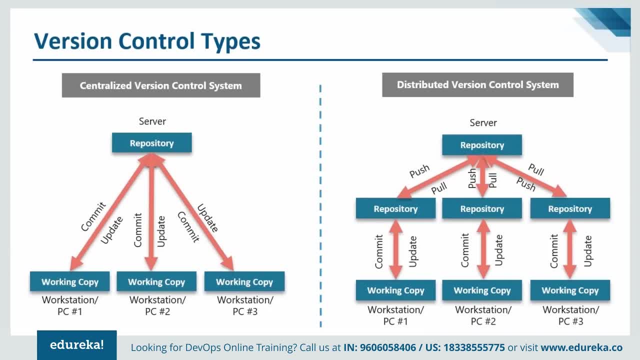 If, at any situation, the central server gets crashed, than the complete data It would be lost. apart from that, since everyone has a full copy of the repository, they can share changes from one another right. So, as I told you before, if they want any feedback before they, 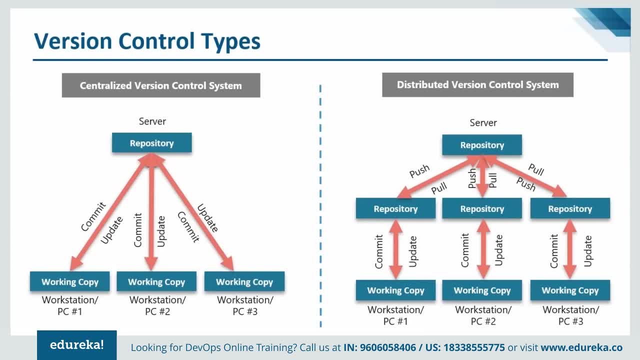 push the changes to the remote repository. they can take the feedback from other developers, make the changes, review it and then push those changes to the remote repository. So, guys, these were some ways by which the distributed version control system was a better option than a centralized version control system. 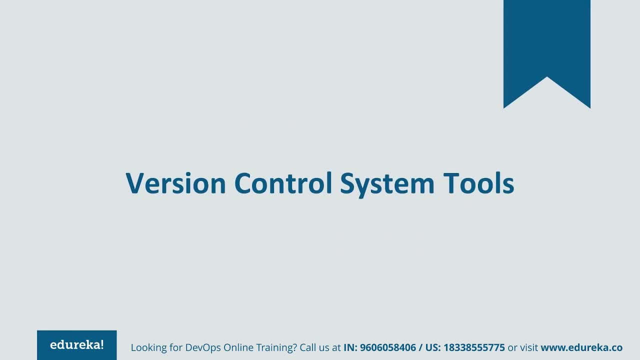 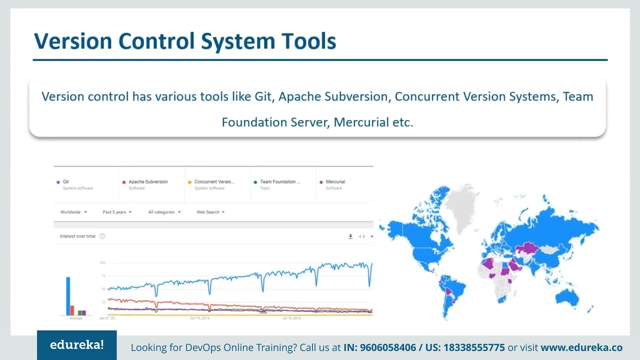 So now that you've got it just about what version control is and what are its various types of systems, Let's look into the tools that offer version controls. Well, the top leading tools in the market are get Apache, subversion, concurrent version systems, team foundation servers, Mercurial. 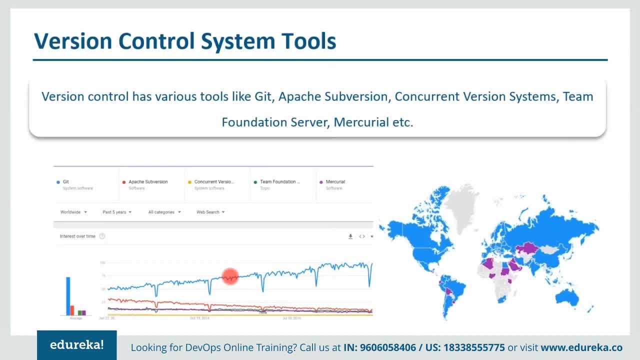 Etc. But out of these tools, we can clearly see on the trends that get wins over the other tools. But why does get win over the other tools? So let's look into it. Well, get offers many features Due to which it wins over the other tools. 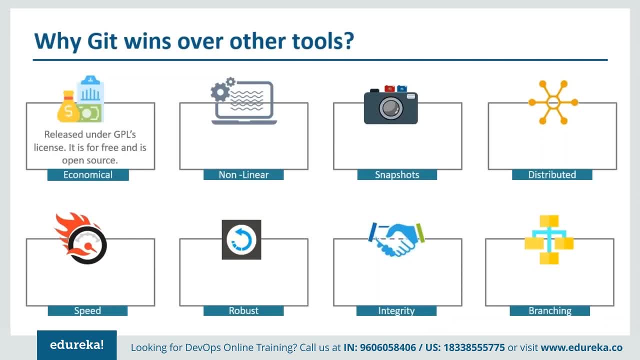 So let's start with the features of kids. So the first feature on the list is: get is economical. So get is released under the GPL's license, It is for free and it is open source. So that makes get economical. next, get is nonlinear. 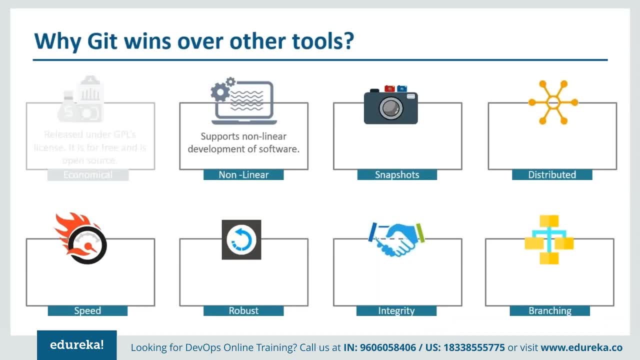 Now when you talk about nonlinear, get supports nonlinear development of software. Now, when you're working with get, get actually records the current state of your project by creating the tree graph from the index. And, as you know, that tree is a nonlinear data structure. It is actually in the form of a directed acyclic graph. 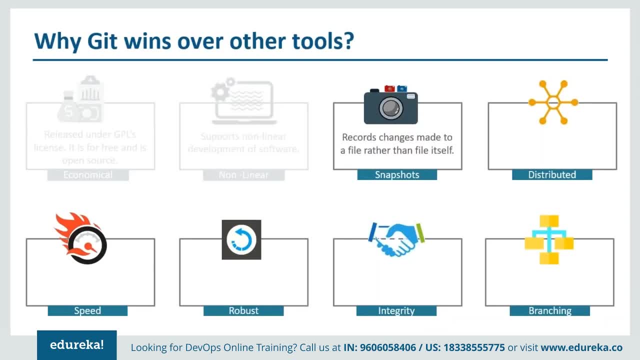 which is popularly known as DAG. next, coming up with a list We have get, providing the concept of snapshots, get records the changes made to the file, rather than changing the file itself. So, as I told you in the example before, if there was a webpage, 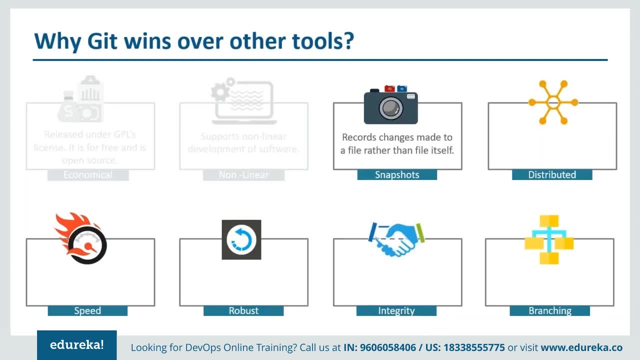 added and there were some photos added in it. get would maintain a snapshot of that. Photos were added in the new web page. now after that in the list we have get offering a distributed architecture. So as get is a distributed version control system. Every user has his own copy of repository data stored locally. 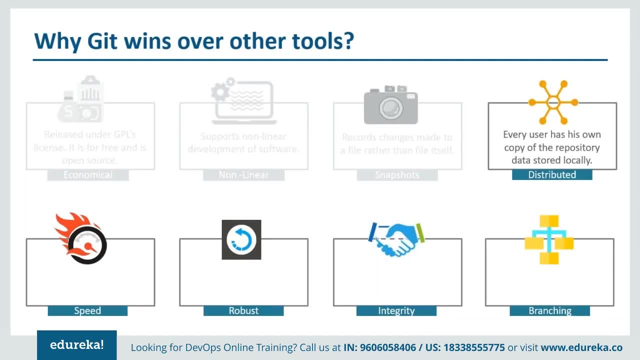 So no changes are made to the central repository unless and until they are pushed from the local repositories. So this is one of the biggest advantages. why get wins over the other tools? next in the list We have get offering speed. Get offers a light fastening speed when compared. 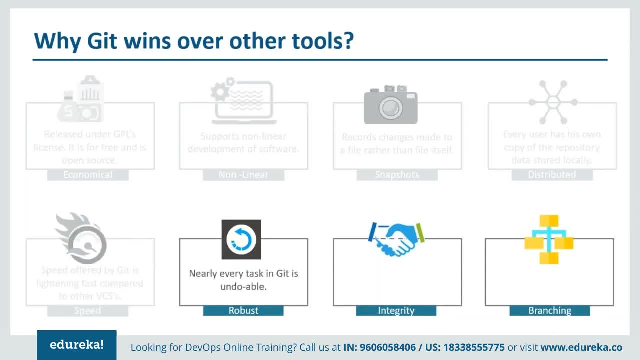 to the other version control tools. Not only does get offer speed, but get is also robust. when I say robust, that is because every task is undoable, So just in case you commit some changes and you want to revert them back, then definitely you can do it. 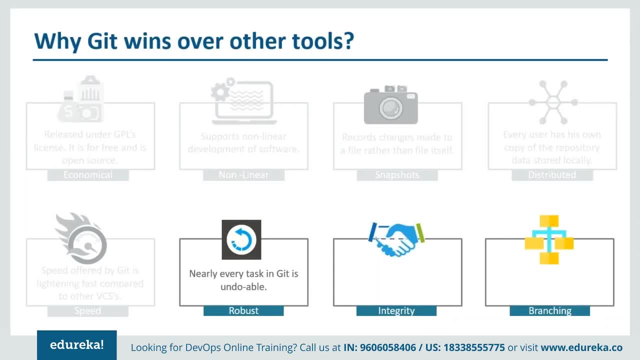 So you can revert back to any action that you have performed, even if it is 10 actions back. So that's how get also offers Integrity. Well, as I said, get records everything, so no changes can be made without get recording it. And finally in the list we have branching. 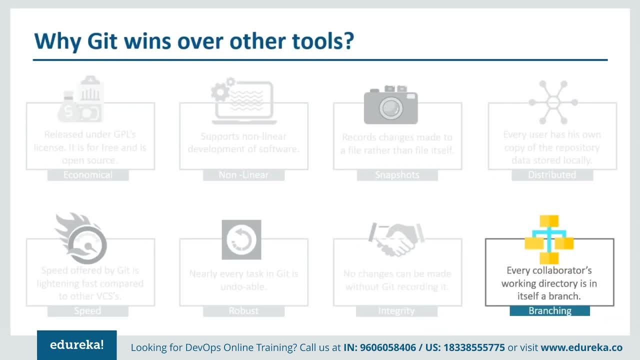 Well, get offers branching. So every collaborators working directory, in itself It's a branch. So get offers nonlinear development, that is, the parallel development, and it also offers branching. So, guys, these were some features of get because of which get wins over the other tools. 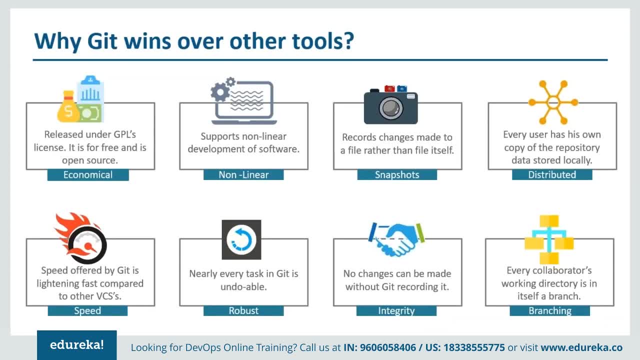 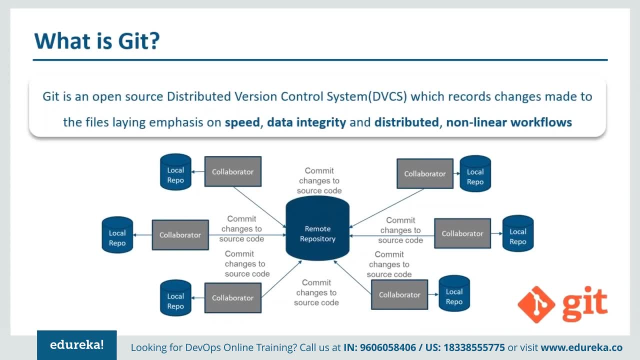 Now that I've told you so many features about get, let me tell you guys what exactly get is. well, get as an open-source, distributed version control system which records changes made to the files, laying emphasis on speed, data Integrity, distributed and nonlinear workflows. So get is the tool that you required to perform all these. 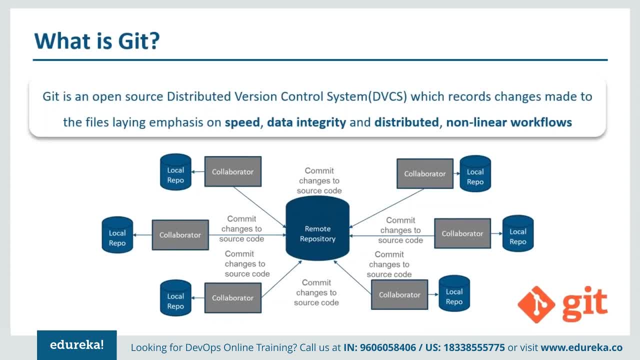 operations. and don't worry, I'll be telling you all about how to perform this operation for using get later in this tutorial. for now, just think of get as the tool that you actually need to do all kind of version control systems. So now let's move on to the workflow of kit. 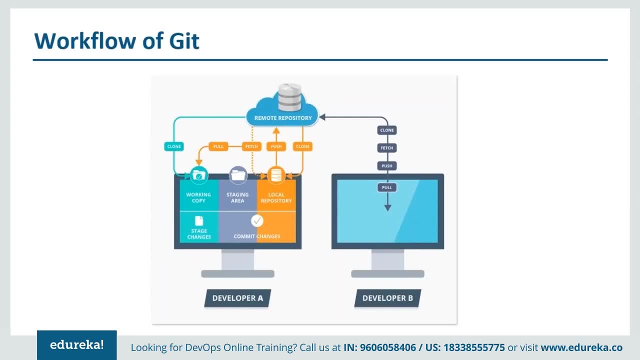 So what do you understand by get workflow? Well, the get workflow is used to manage your project effectively. So, basically, if you work with a set of guidelines, then it obviously increases your consistency and productivity. now let's discuss each and every component in the get. 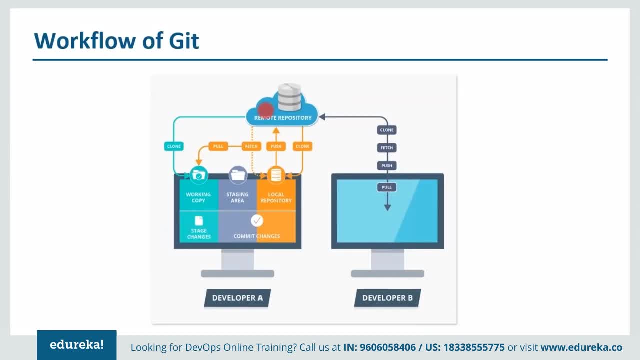 workflow, starting with the remote repository. remote repository is the server where all the collaborators upload the changes made to the files. So all the changes that each and every collaborator makes is uploaded to this remote repository. Next we have the local repository, as I mentioned before. 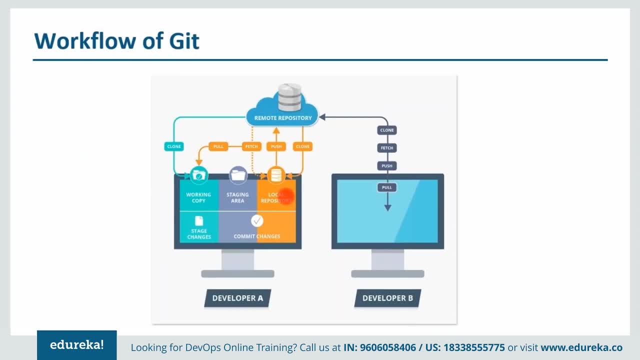 the local repository is the user's copy of version database. So the users access all the files through the local repository and then make changes. once they have a set of changes, they push the changes to the remote repository. So if there are n number of people working on an application, 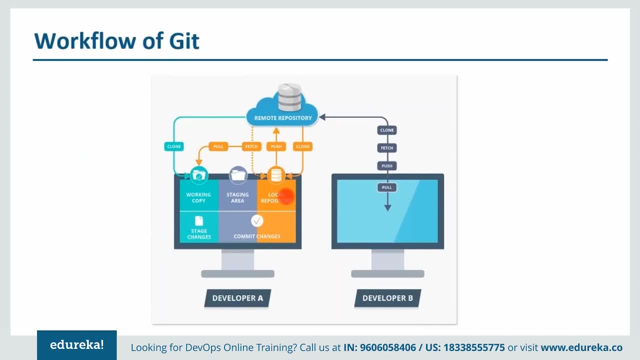 then there are n local repositories and then each one of them can make changes in the local repositories. Once they are done, They can push all these changes to the remote repository. Then we have to working copy. the working copy is nothing but the users Active Directory and this the user modifies. 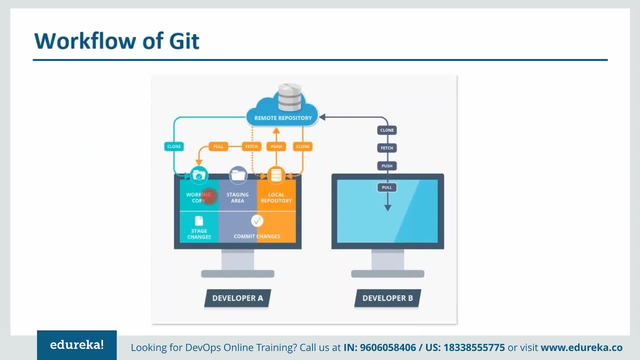 the existing files and creates new files in the space. So basically, this is the area where the user makes changes, So get tracks these changes and compares it to the local repository. Next we have the staging area. So the staging area Is a place where all the modified files marked to be committed. 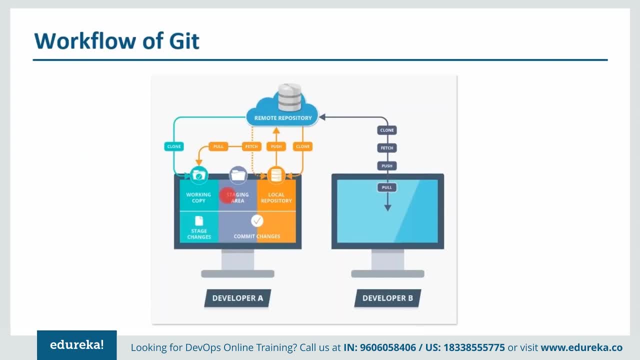 are placed. So, basically, once you make the changes and then you want to commit this changes, before committing you put them into the staging area. So basically, you can visualize this place as the place between the working copy and the local repository. now coming to the commands used to perform these actions, 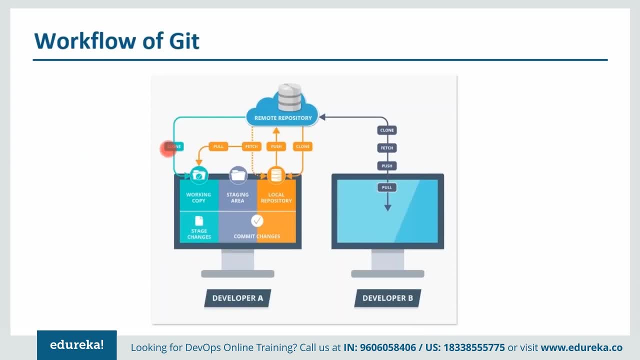 and get. the clone command creates a copy of an existing remote repository inside the local repository. So basically this command is used to make a call to create a copy of the existing remote repository. So anytime you want to create a copy of the existing remote repository. 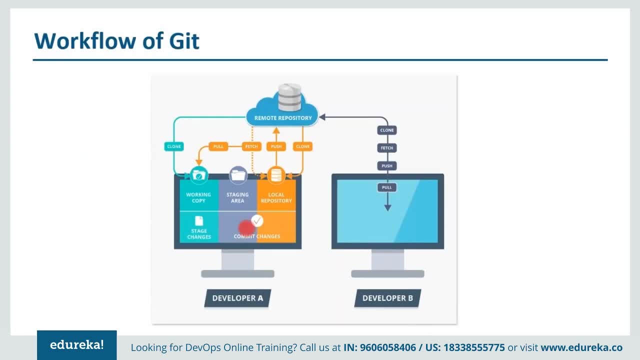 then you use the clone command. next you have to commit command. the commit command commits all the files in the staging area to the local repository. after that we have the push command. the push command pushes all the changes made in the local repository to the remote repository. 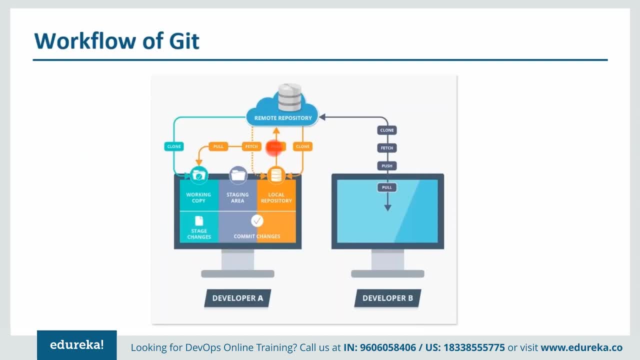 So anytime you have a set of changes ready, then you can use the push command to push all the changes from the local repository to the remote repository. After that we have the fetch command. the fetch command collects the changes made at the remote repositories and copies them to the local repository. 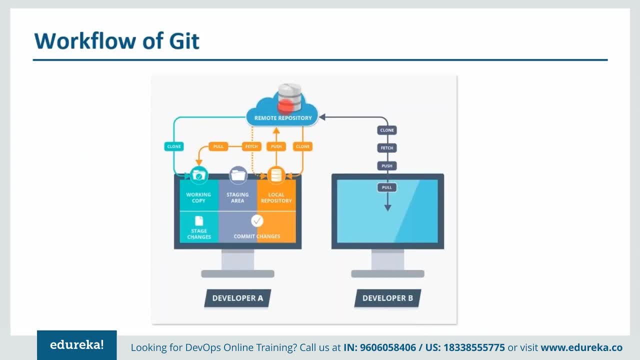 So any changes that you make in the remote repository, the fetch command copies these changes and puts them into your local repository. Well, let me tell you that this command doesn't affect our workspace. that is a working copy. Now, the pull command is similar to that of the fetch command. 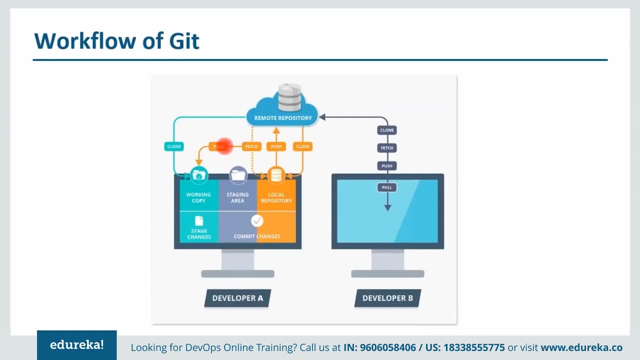 It gets all the changes from the remote repositories and copies them to the local repository. So basically, pull merges those changes to the current working directory. So, guys, I hope that you're clear with the components for the get workflow and the commands used for it. 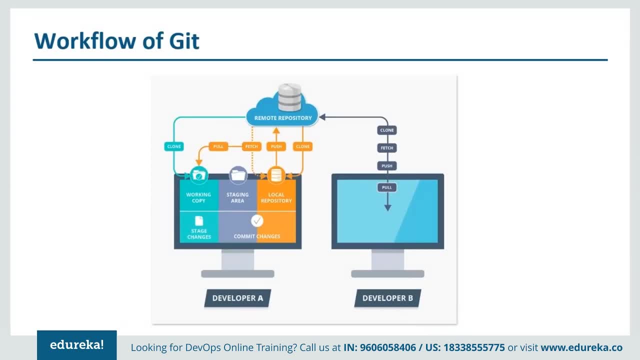 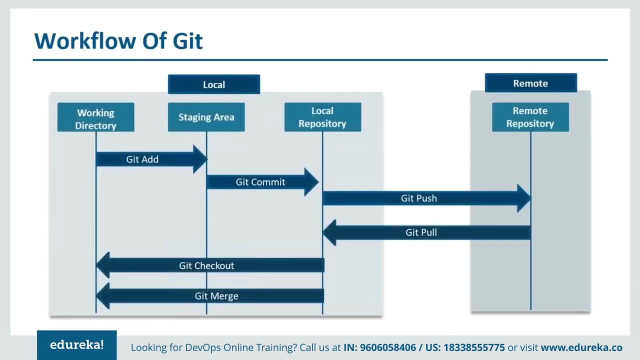 Okay, so most of you say yes. So now that you have a basic idea of get workflow components and the commands use, let's discuss the workflow now. So, as you can see the diagram on the screen, I'm going to explain the workflow of get through this diagram. 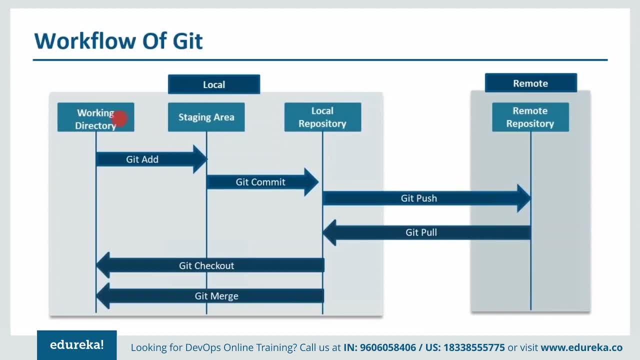 So suppose I am a developer and this is my working directory. Now what I want to do is I want to make some changes to the local repository. So, since it is a distributed version control system, I have my local repository as well. Now what I'll do is I'll perform the get add operation here now. 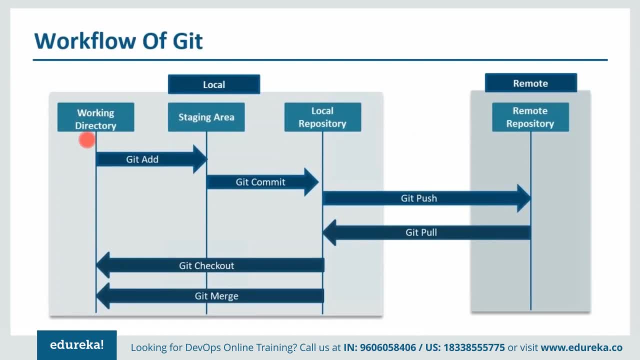 because of this get add operation, whatever was there in the working directory has been put into the staging area. Now you can visualize the staging area as the place between the working directory and the local directory. Once I have all my uncommitted changes in the staging area, 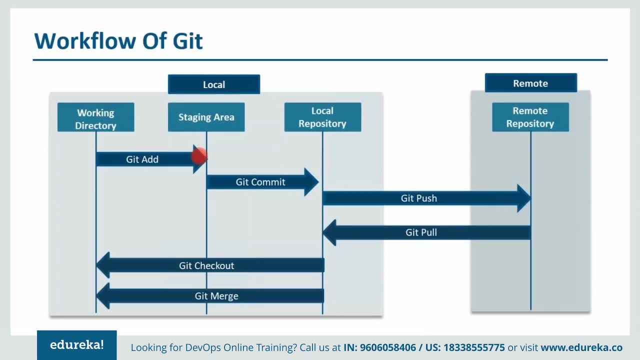 I want them to get committed into the local repository. So for that I'll perform the get commit option and then I'll commit all the changes to the local repository. and once I'm done with all the set of changes I'll go ahead and I'll push these changes. 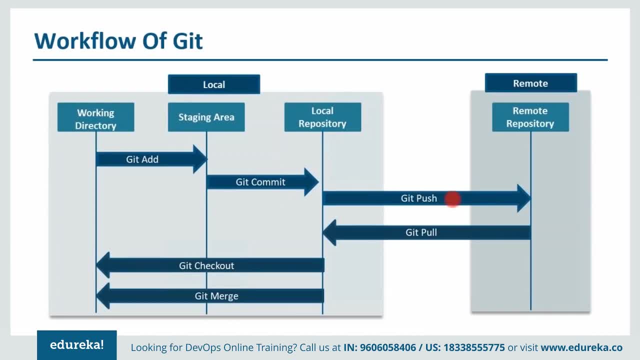 to the remote repositories as well. after that you can perform the get pull option to add whatever is there in your remote repository to your local repository, and then you can perform the get change Checkout command to add it to the working directory as well. It's really simple, right. 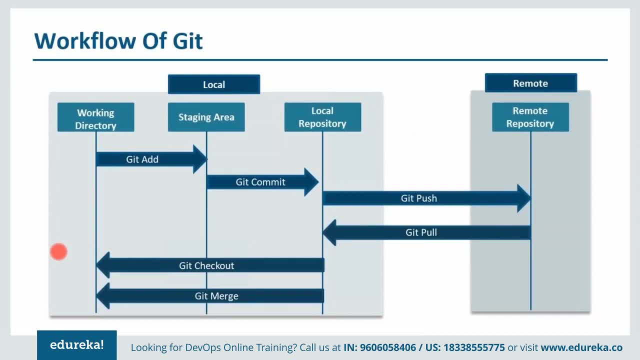 So you just have to make changes in your working directory, add them to the staging area and then commit them to the local repository. Once you're done, you just push all these changes to the remote repositories and, whenever you want, whatever is there in the remote repositories. 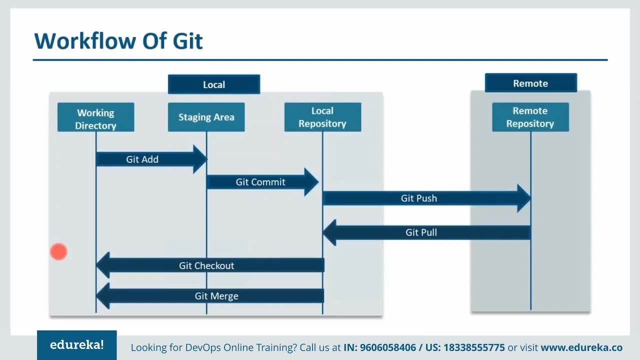 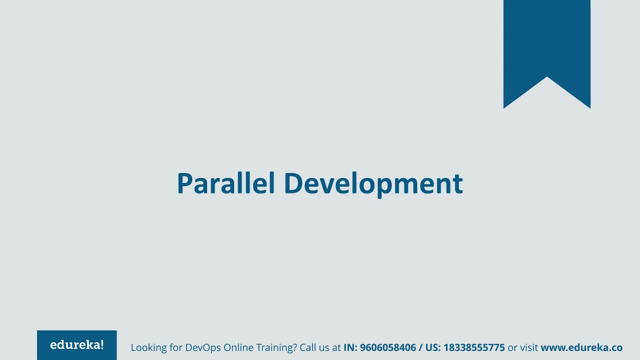 you just simply pull whatever is there in your remote repository to the local repository and then also copy these changes to the working directory by using the get checkout command. So, guys, that's how simply get works. Get not only provides a simple workflow, but it also provides parallel development. 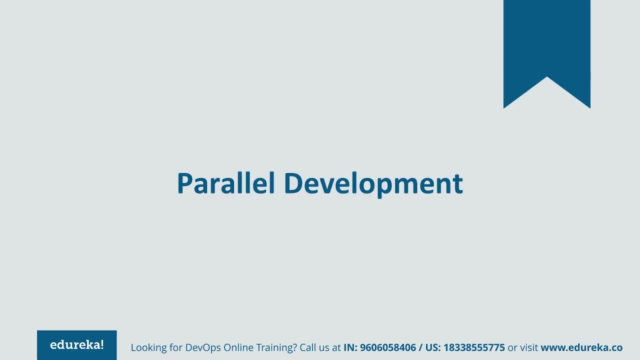 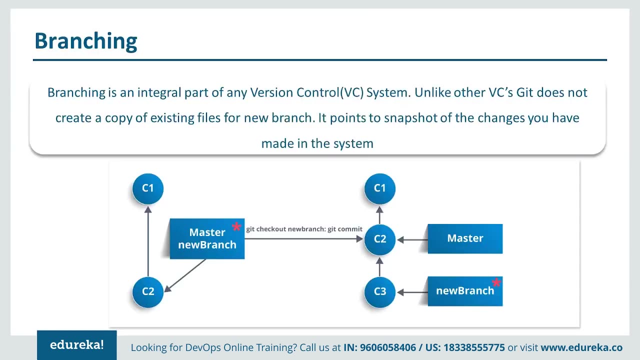 or nonlinear development. Well, when I say parallel development, I mean various operations that get provides, well, get provides stream in operations: branching, merging and rebasing. with rebasing- various other concepts come like reverting and resetting. So first let's talk about branching. 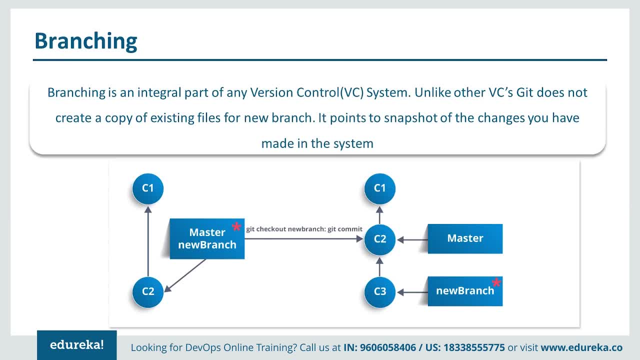 Well, in simple terms, how do you understand branching? Well, you can just assume it like a tree. A tree has various branches and it has one master branch, that is the stem. Similarly, you can think of branches like a pointer to a specific commit. 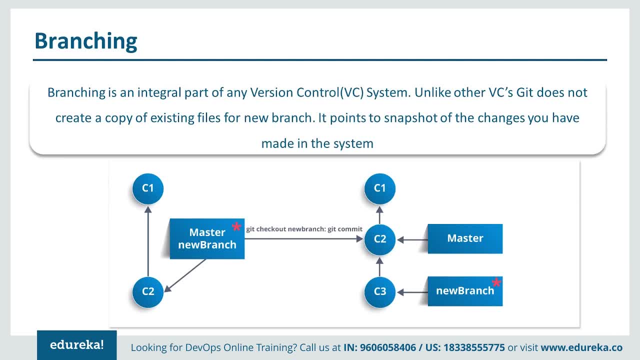 Let's say that you have made changes in your main branch. and now remember, whenever I say main branch, I'm talking about the master branch, right? So the master branch is our main branch. Now this master branch contains all the codes. So let's say you're working on the master branch. 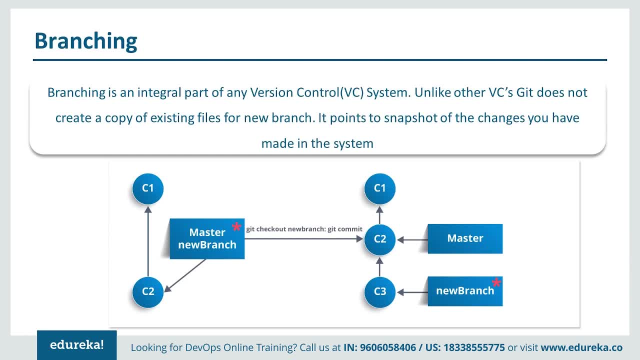 and you've just made a change and you've decided To add some new feature onto it. So you want to work on the new feature individually and you don't want to interfere it with the master branch. So for that, if you want to separate the master branch, 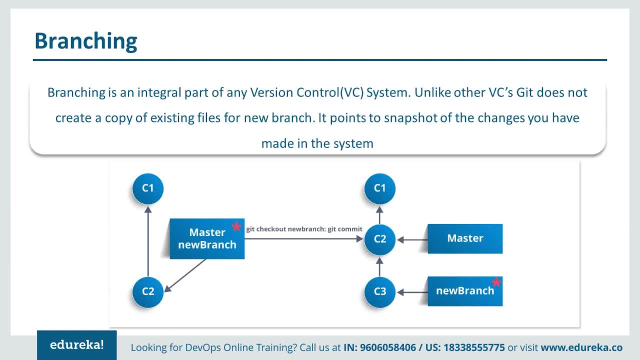 from the feature, then you can actually create a branch from this comment. So, basically, if you want to work on any feature specifically and you do not want the master branch to get involved with it, then you create a new branch on that comment. All right, so there are two kinds of branches. 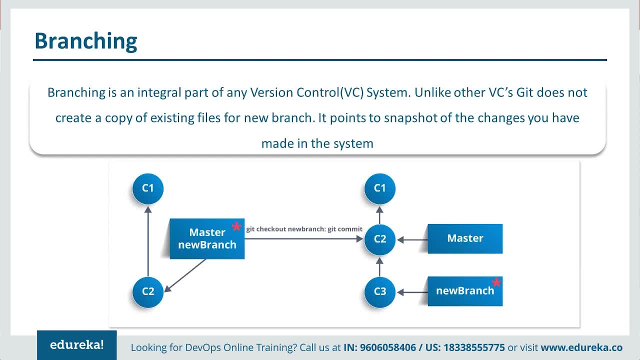 that is, mainly the local branches and the remote tracking branches. So your remote tracking branches are the branches that is going to connect your branches from your local repository to the central repository, and the local branches are something that you only create in your workspace and that is only going to work with your files. 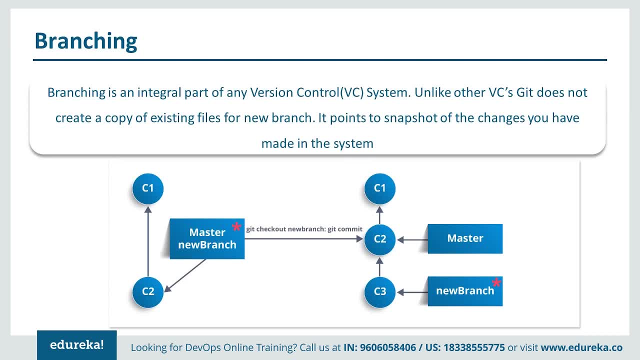 in the local repository. So obviously branching is an integral part of version control system. Unlike the other version control systems, get does not create a copy of existing files for a new branch. It just points out to the snapshot of the changes you have made in the system. 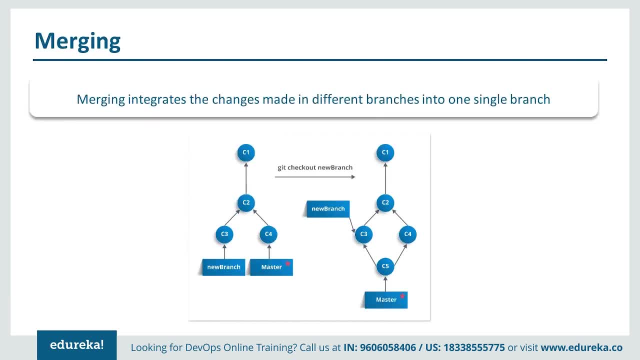 So it's really simple. So now, moving forward to the next operation. The next operation we have is merging. So now, if you're creating branches and you're developing a new feature and you want to add this new feature, then you have to do an operation called merging. merging combines. 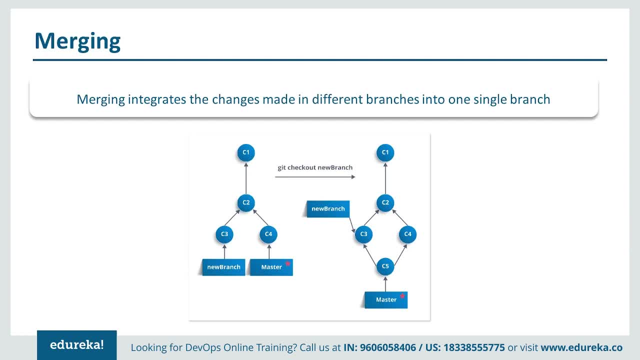 the work of different branches all together and it's really important that after you've branched off from your master branch, always combine it back at the end after you're done working with the branch right. So what I'm trying to say is, once you create a branch, 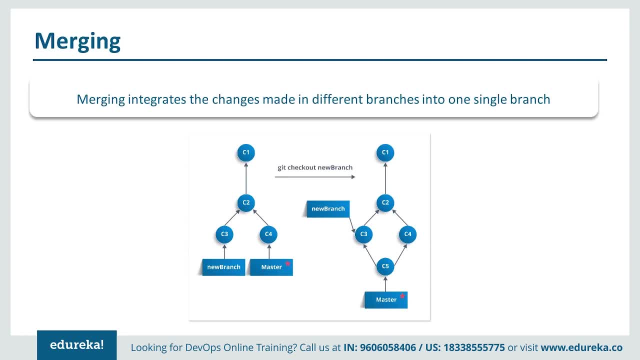 and then you're done working with that particular branch. you have to merge it back to the master branch. So in simple words, merging integrates the changes made in different branches into a single branch. So it's really simple. So just imagine a master branches, 5 to 6 new branches. 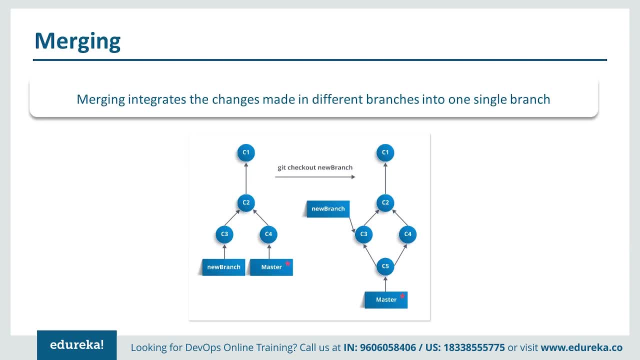 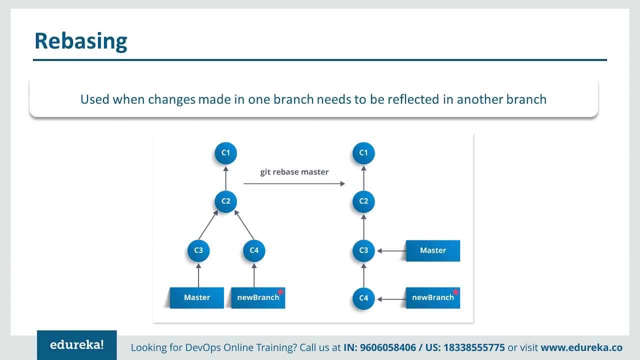 So once you're done working with all this 5 to 6 branches, you just have to merge them to the master branch. Now, next in the list, We have rebasing. rebasing is also another kind of merging, so the standard rebase is: 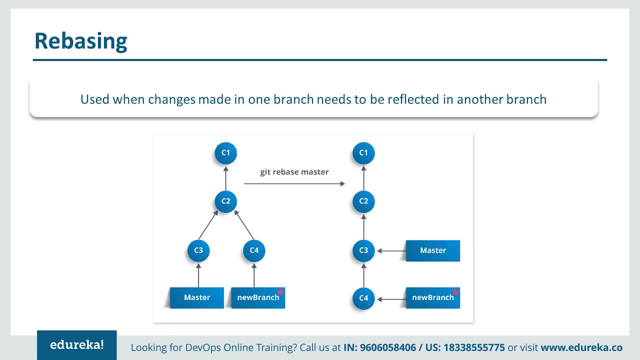 that it actually solves the same problem as merge, and both of these commands are designed to integrate changes from one branch into another, and the fact is that they just do it in different ways. Now, what does rebasing me if you see the workflow diagram here? 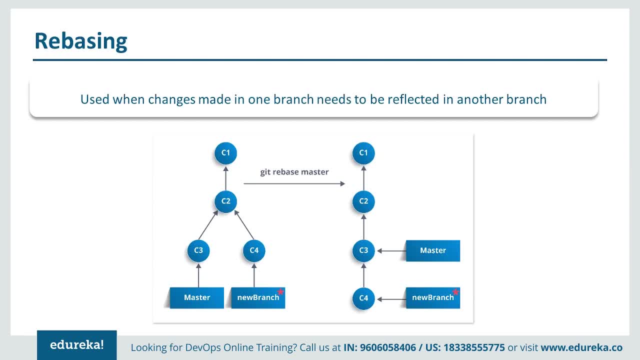 you've got a master branch and you've got a new branch now. So when you're rebasing it, what it does is you can see in this workflow, So it's got a new branch and your master branch, and when you're rebasing, 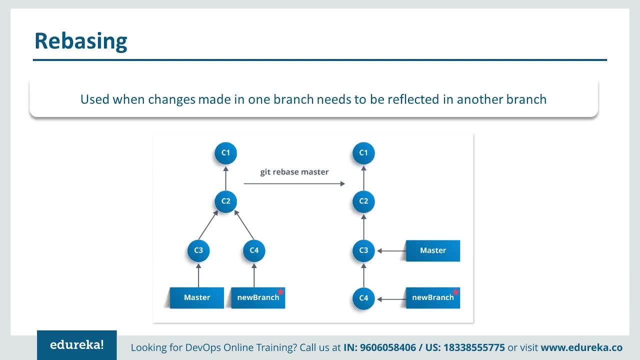 it instead of creating a similar commit which will have to parent commits. what rebasing does is that it actually places the entire comment history of your branch onto the tip of the master. Now you can ask me: why should we do that Like? what is the use? 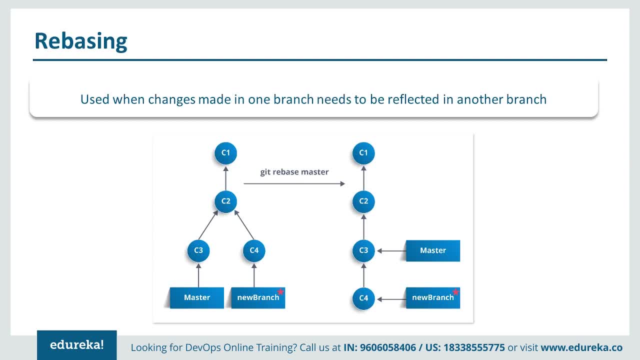 or what is the major benefit of using rebase? So basically, rebase offers you a much cleaner project history and also, rebase is used when changes made in one branch need to be reflected in any another branch, So any change that you make in any particular branch. 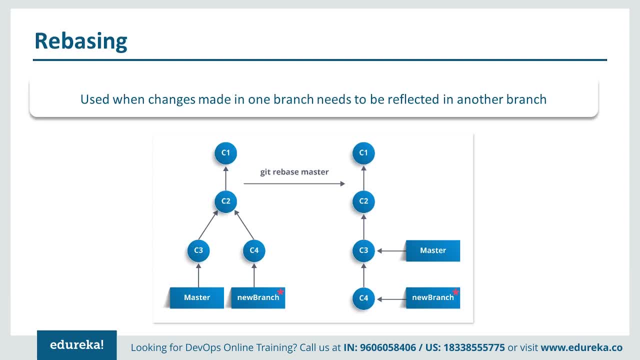 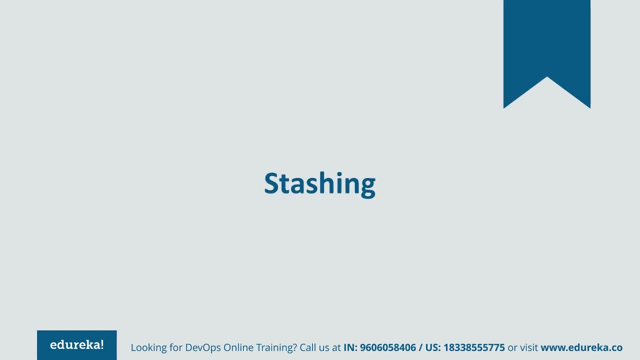 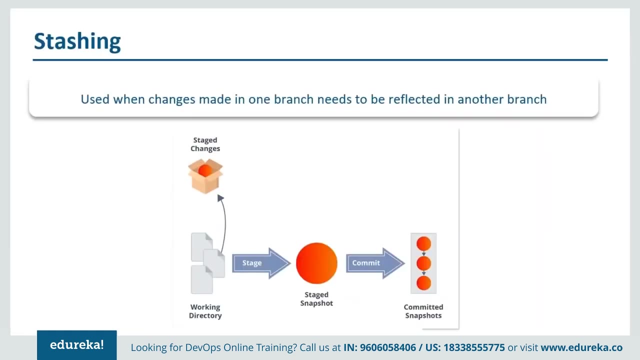 and that change needs to be reflected in any under the branch, then you need rebase. Now that you've understood what parallel development is and what get offers regarding the pallet development, Let's move on to another important operation about get, that is stashing. now, get stashing is a way. 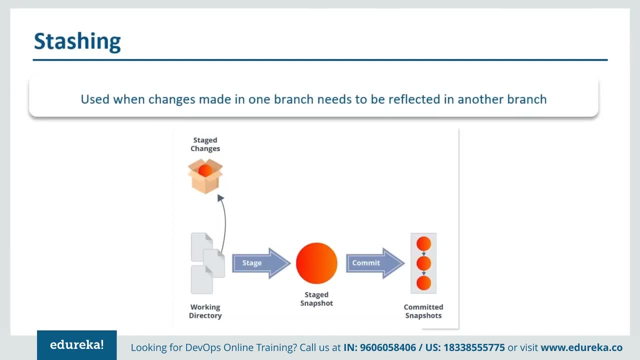 of creating a checkpoint for non-committed changes. It saves all the changes to a temporary locations so that the user can perform Other tasks, such as switching branches, reverting, Etc. These changes can be reapplied anywhere. So, as you can see in the diagram on the screen, 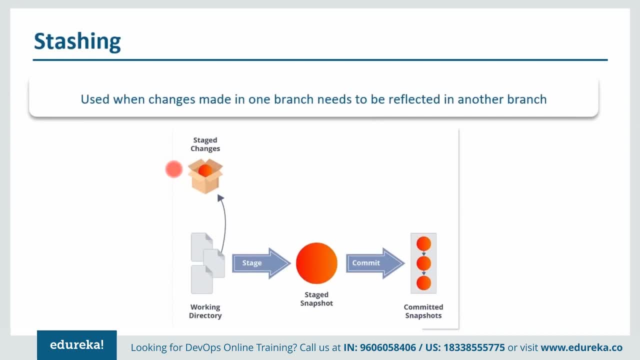 this is the temporary location to which the user can save all the uncommitted changes and then perform actions such as reverting and switching through branches here. So whenever the user wants some changes which are stored in the temporary location, he can just apply these changes anywhere. 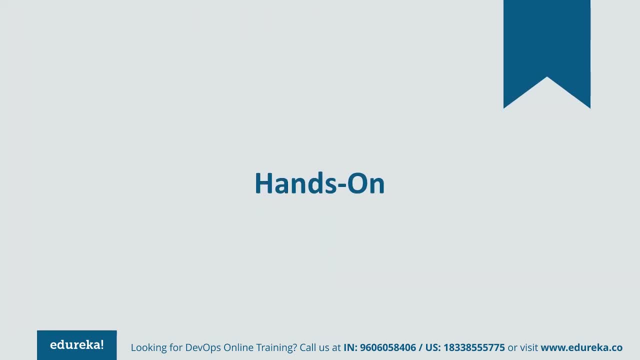 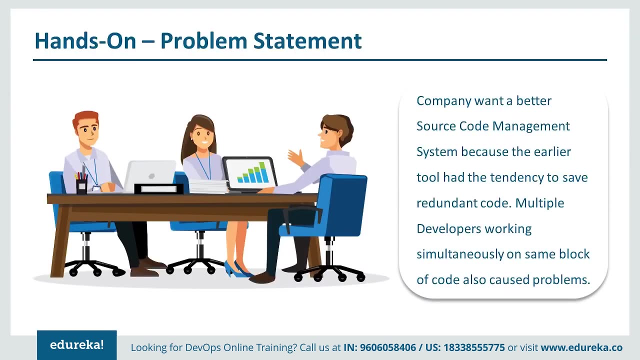 Now that I've told you so much about version control systems and get and different operations in get, let's move on to a hands-on part where we'll be performing all these operations. So we have a company with three developers are working. now They want the company to have a better source code management. 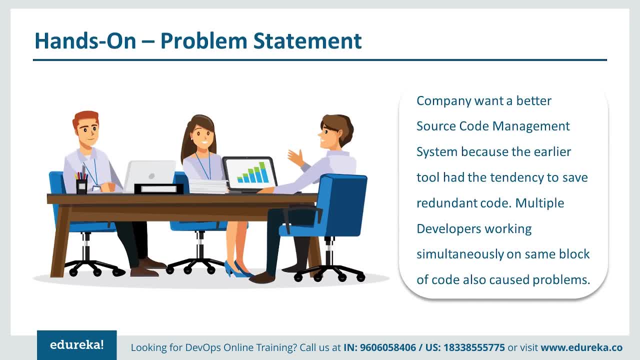 So whenever I say source code management, I'm referring to the version control system. These developers want a better source code management because the earlier tool had the tendency to save redundant code, So they did not want redundant code in the system. So they faced issues such as men, multiple developers. 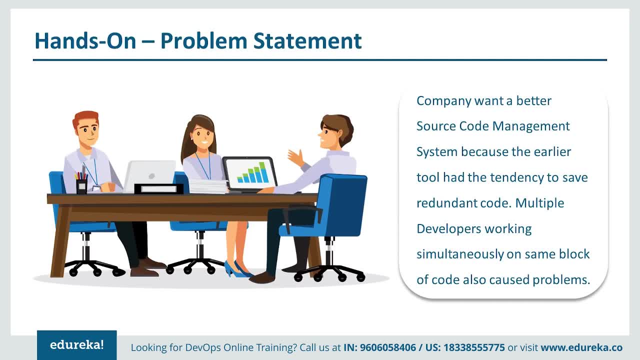 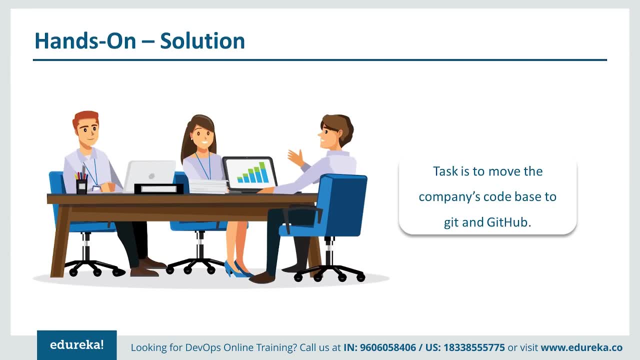 were working on the same block of code. There were a lot of changes happening and nobody knew who was making so. the solution to this problem is to move the code of this company to GitHub and use get. so how do we do that? Well, we're going to create a local repository. 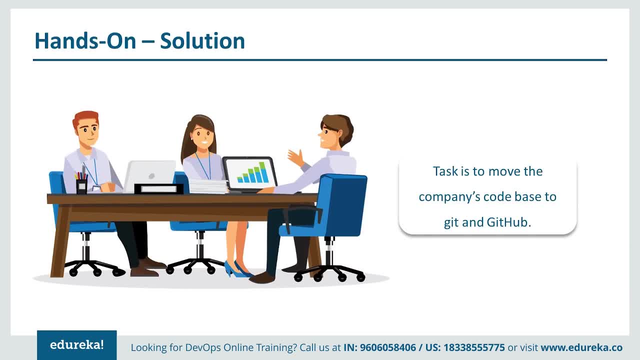 and then move the entire code base into it. Then we're going to create a new branch for this new feature that you want to add to the application. Then we will merge back this created branch with the master and then we'll create an remote repository. 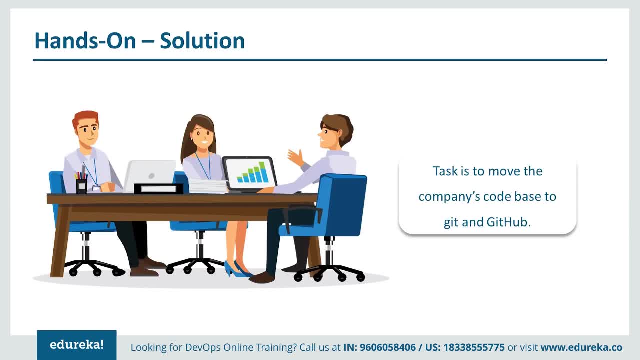 after that We'll see how rebasing and stashing is performed and then finally push this local repository to the remote repository. Okay, So now let's get started with the hands-on. All right guys? So let me go to the Linux operating system. 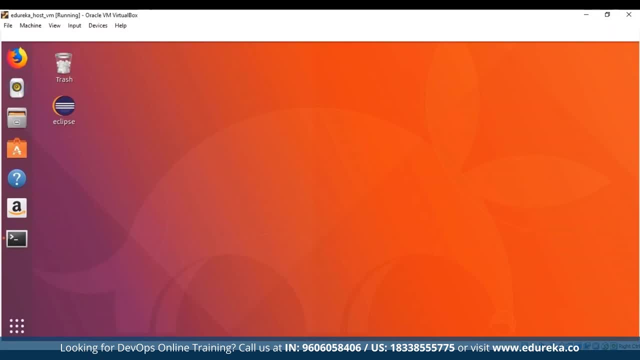 where I've installed my git. just in case you want to know how to install git, then you can refer to the git installation video, which is mentioned in the description box below. So now let's get started with the hands-on. So our first task is to create a local repository. 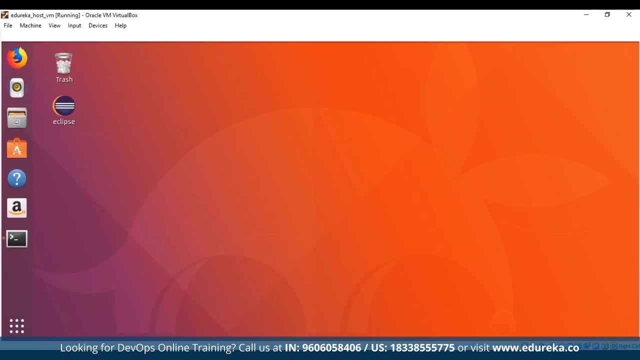 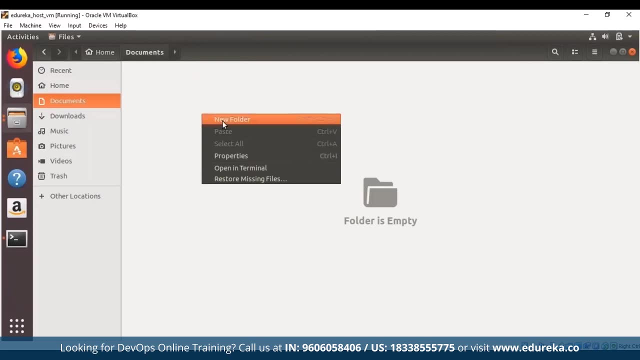 on the local machine and then also to create a repository in the GitHub account. Let me just create a repository. So let's say I create a new folder with the name get tutorials hands-on, And then I go back to the GitHub account and then I create a new repository. 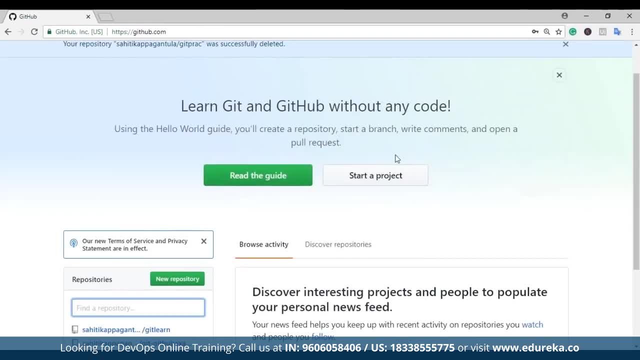 So this is my GitHub account. after creating the local repository on your local machine, You also have to create the remote repository on the GitHub website. So, guys, this is my account. If you want to log into the githubcom, you just have to type githubcom. 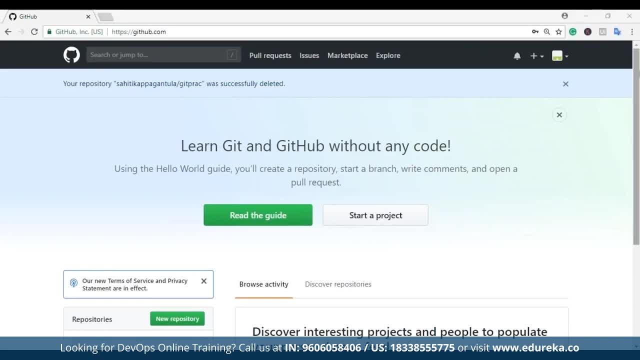 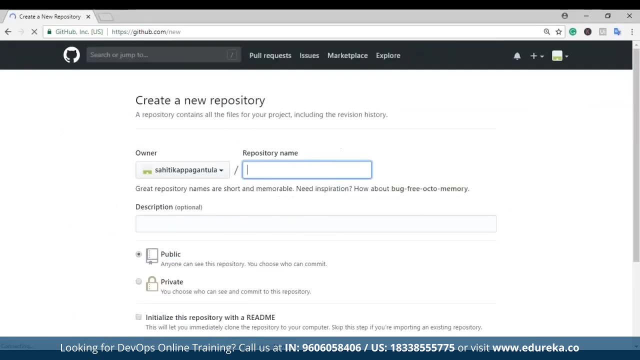 and then you have to fill in the sign-in details. Once you're done with that, you'll be redirected to this page and over here you can add new repositories. So let me just add a new repository. So if to give the repository name, 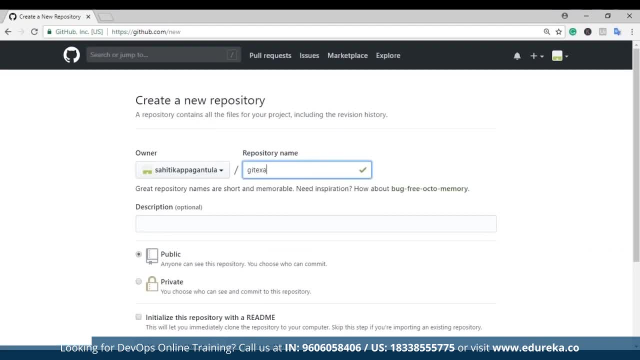 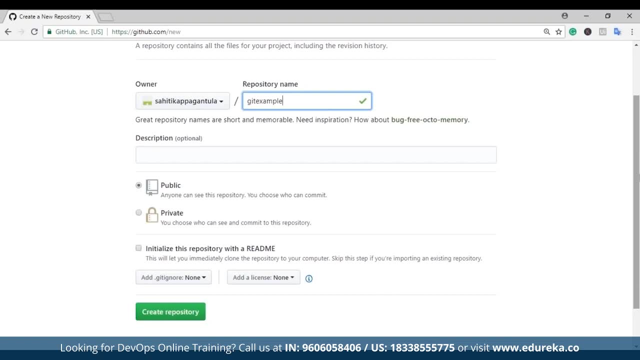 so let's say I give the repository name, as get example, and then I'll choose a repository to be public. If I want this to be private, then I have to buy a license. I'll just choose the option public and then I'll click on create repository. 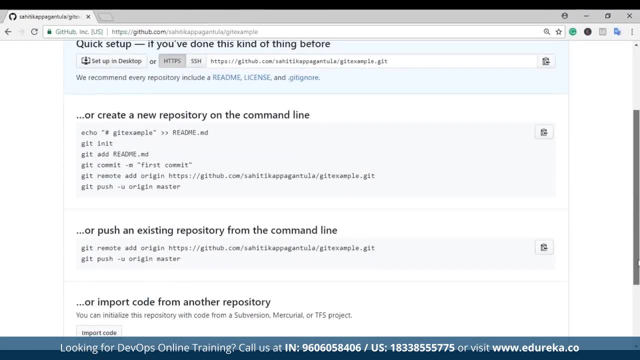 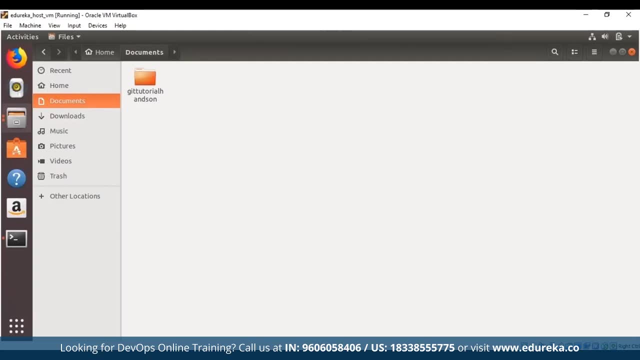 So you can see that my repository has been created here. Now what we have to do is we have to make the changes on our local repository and then we have to come at this, changes to our remote repository. So now let's get started. Let me go back to my local repository. 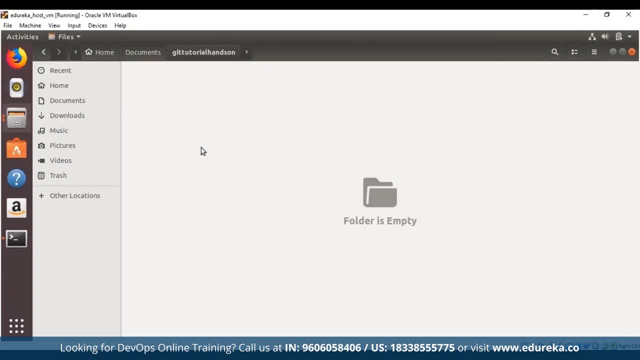 and over here I'll put in the code base for the company. So let me just put in the code base. so let me just go back to downloads, Copy this, Go to documents and let me paste it here. So that means all the source code. 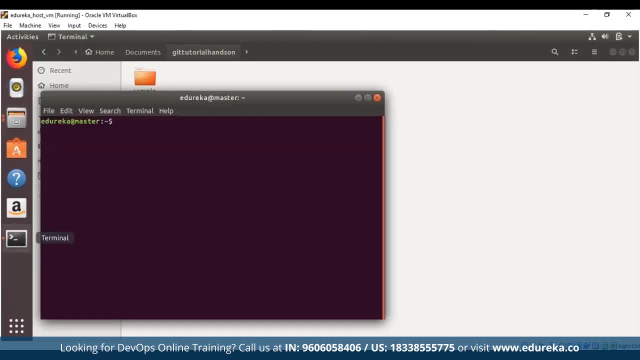 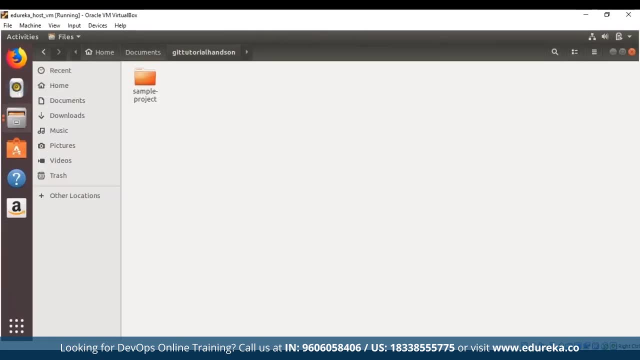 for this company is present in the local repository. Now what we have to do is we have to make changes in this repository and then come in the changes to our remote repository. So for that, let me just go to this folder. So for that, let me just open the terminal. 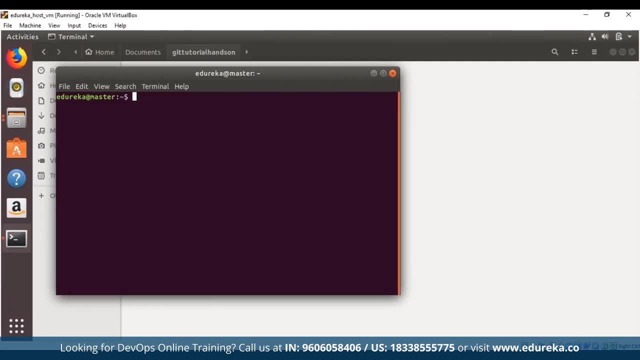 So I'll open the terminal now. in this terminal We have to go to this particular local repository, So let's just type in the path name. Once you go into this folder, let's just list all the items that are present in this folder. 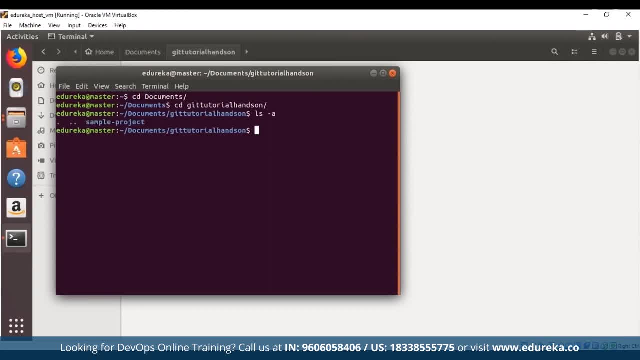 Well, you can see that the sample project, that is the sample code for the company. So now let's go to this particular folder and see what all is there in it. So let's use the command Ellis, hyphen a, which will basically list all the files. 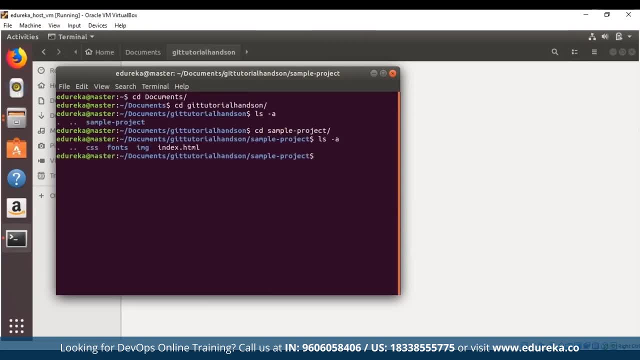 and folders that are present in this particular folder. So you can see that it has folders for CSS, fonts, image, and it has a particular file that is indexed, or HTML. All right, So now what we have to do is we have to initialize, get on this particular folder. 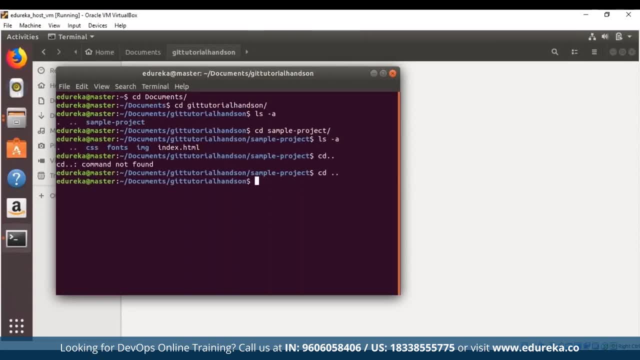 So let's just go back to this get tutorial hands-on folder and then let's initialize get here. So for that I'll use the command get in it. So this command will basically initialize get for this particular folder. Well, you can see an output. 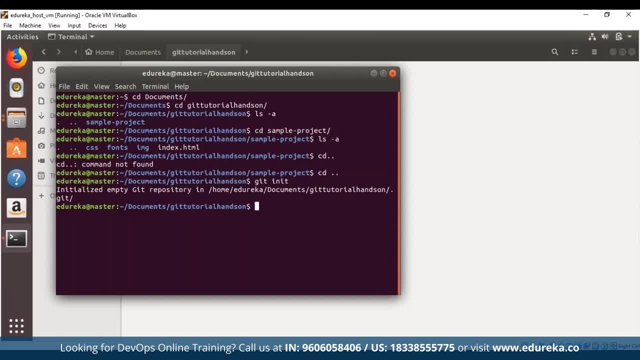 that initialized empty get repository in this particular folder, right? So basically this is a working copy. Now what we have to do is we have to basically add this folder to the staging area. So let's just use the command get add to add this folder. 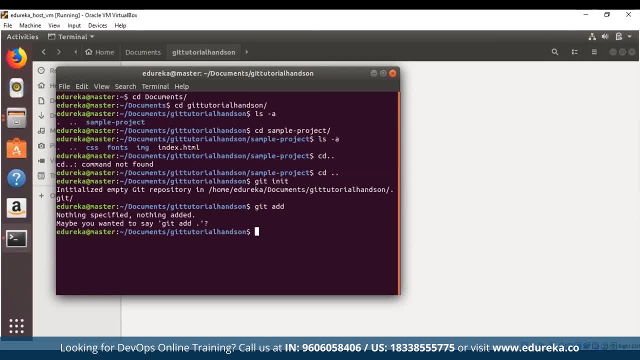 So so as you can see that we have to use the file name to add the folder, So we have to be really specific, right? So we'll use get add space dot. dot means all the files and folders in this particular gift tutorial hands-on folder. 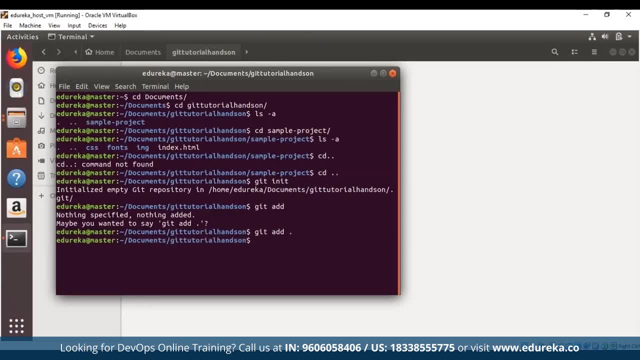 would be added to the staging area. So that means our folders have been added. now we have to come at it. So for that, if you want to come at the folder, then you have to just use get commit. So when you use the get commit command, 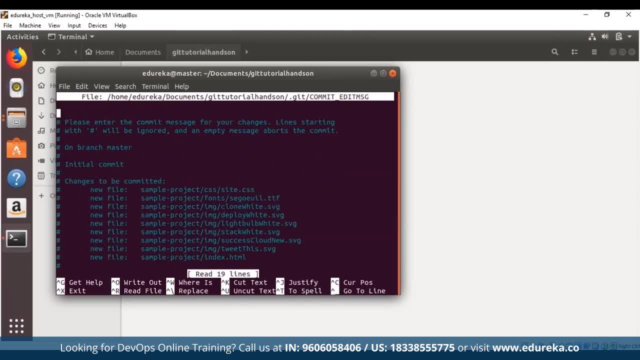 you can see that it asks us to enter a commit message. So let's just say I enter the commit message, as this is the first commit commit for the project, And then I'll press on control X and I'll save this file So you can read the first. 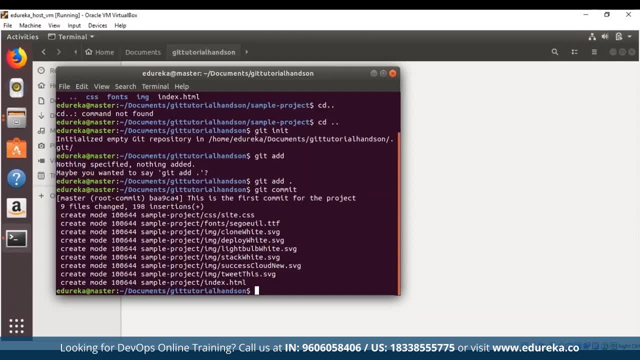 commit message. as this is the first commit for the project right now, if you want to check on which branch are you working and if there's anything that you have to commit or not, you just have to type in the command get status. So with this command, 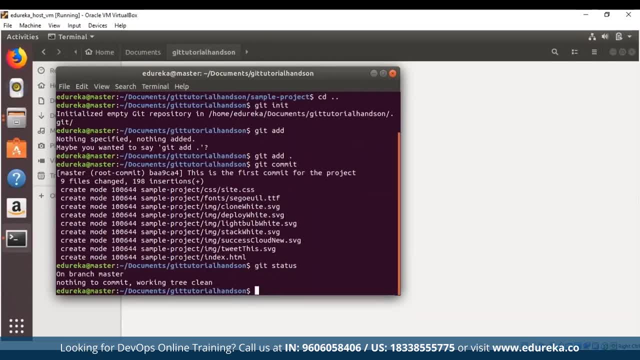 you'll know that you're working on the master branch and you have nothing to commit Now. if you want to know how many comments have happened and what are the changes that have happened in the commit, then you just have to type in the command get log. 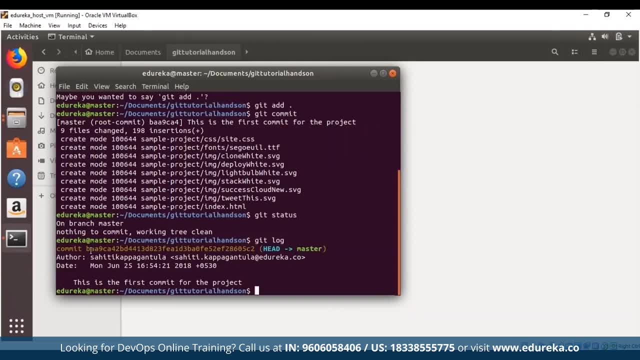 So you can see that there's a particular commit ID associated With each commit, and then you also know the author, date, time and what has been changed, right? So anytime you enter a commit message it will consist of what has been changed. So the comment message will basically tell you.